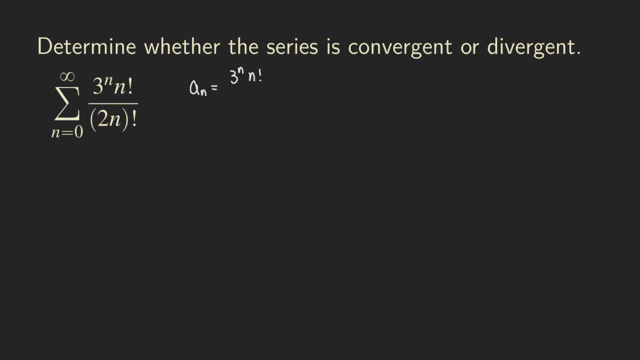 that's showing the problem. So we are going to get three to the n and then n factorial. And then what do we get in the denominator? We have two n and then factorial. Okay, so now what is the next turn? The next turn is the ace of n plus one. 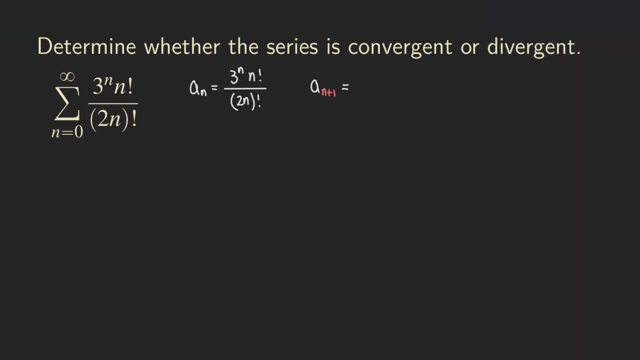 Okay, So for the ace of n plus one, we are going to have three to the n plus one. So wherever we see the n, we are going to replace it by n plus one. then we are going to get the n factorial. 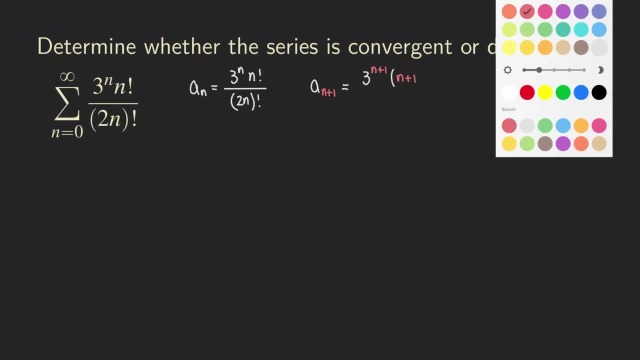 So that's also being replaced by n plus one, then factorial And then from there, there in the denominator, we are going to have two and then now this one. we need to be a little bit more careful when we put down the n plus one. we actually need to put a pair parentheses around. 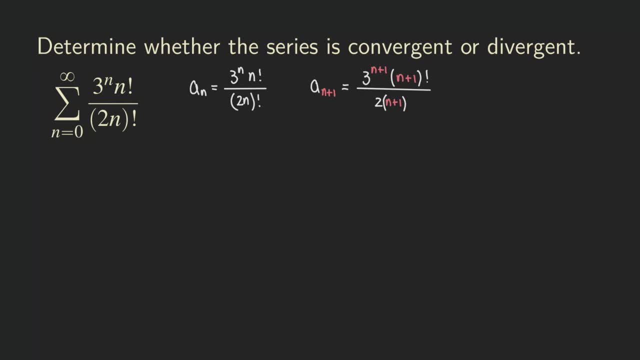 the n plus one, because the two will get distributed to the n and the one. and then on the other side, there is the factorial. okay, for this one we probably need to do a little bit of simplifying before we will put it in the uh, before we put in the ratio, the limit, okay. so 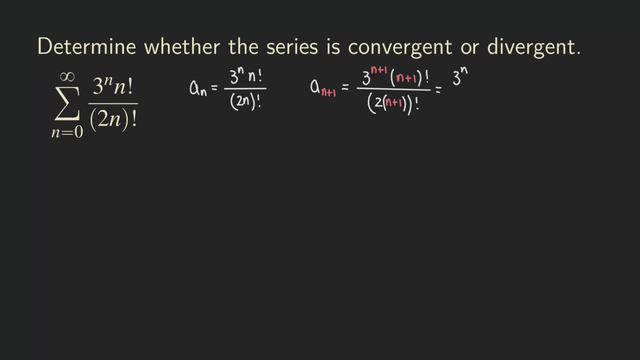 we can write it as 3 to the n and then times 3. so we are just using rules of expellance to break this 3 to the n plus 1 apart into 3 to the n times 3 to the first power. then for this n plus one. 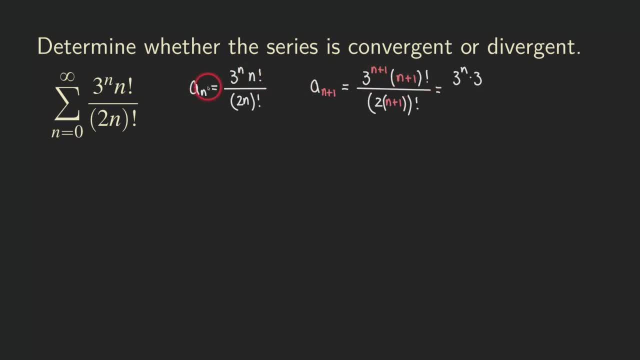 factorial. if you see that there was a from the previous turn, there was an n factorial here. this is really just having an extra factor of that n factorial. So we can write this n plus 1 factorial as n plus 1 times n factorial. And then now we get to the denominator. So for the denominator. 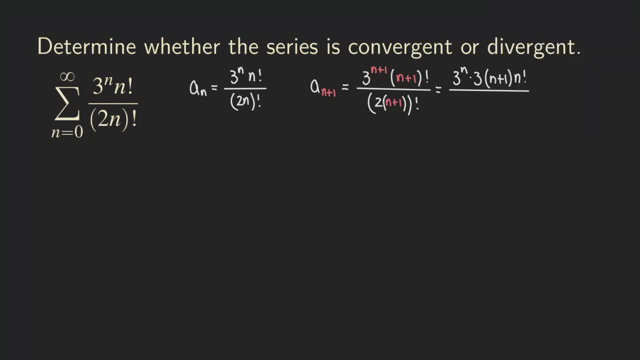 we are going to: first let's just realize that this is actually just 2n plus 2.. And then, instead of writing that, let's just write down the whole thing. So it's actually just 2n plus 2, and then factorial, So to expand this one, we are going to write it as what We are going to write. 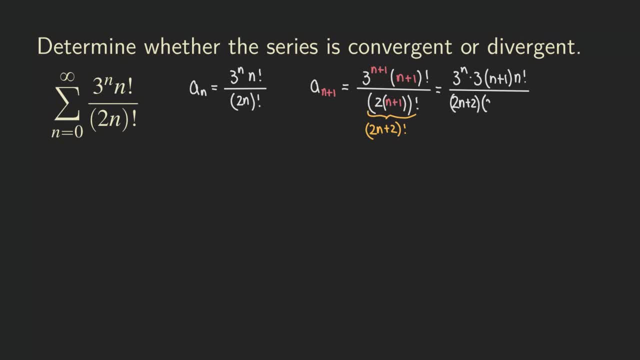 it as 2n plus 2 and then 2n plus 1, because that's the next factor, And then we are going to get the 2n and then factorial. So the fraction line is too short, so it doesn't cover that. So let me. 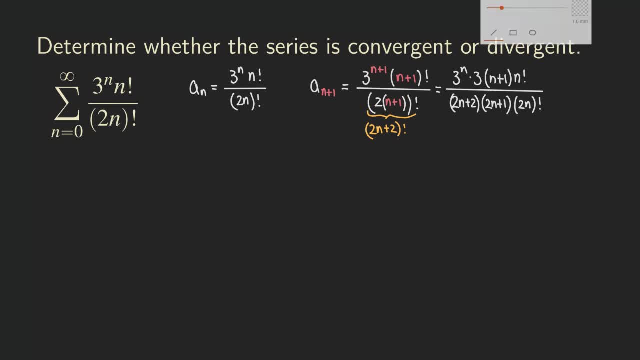 just erase that And then let me re-draw it so that it will cover all that. Okay, so now that's good. Okay, so what do we do next? We are going to start taking the limit of the ratio of the two. 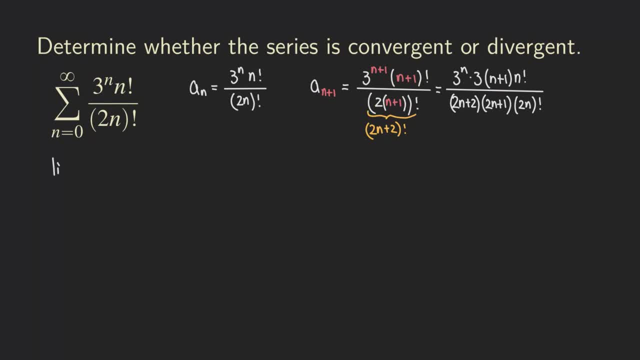 terms. right, So we are going to take the limit. as n approaches infinity, We have the absolute value of the a sub n plus 1 over the a sub n. Okay, so what are we getting here? We are going to, we are going to get absolute value here: 3 to the n times 3 times n plus 1 times n factorial. 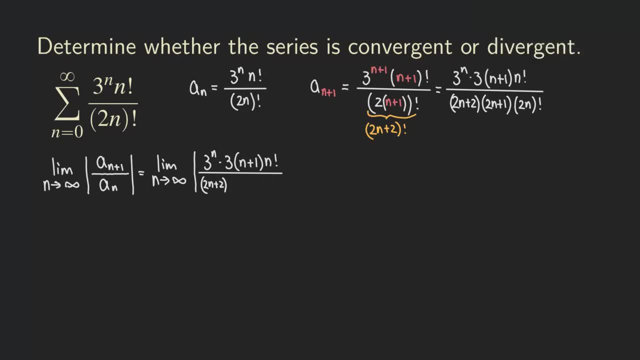 Then from there we are going to get 2n plus 2, and then 2n plus 1, and then 2n factorial, and then times. Now when we multiply, we are going to multiply by the second half, So we are going to get 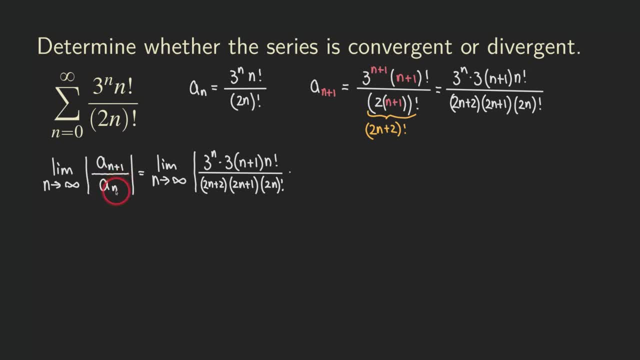 by the reciprocal of the a n, because we are dividing by a n, right? so we are going to put the reciprocal of the a n here. which becomes? what does it become? it becomes what? two, two, two n, factorial, okay. and then what do we get in the denominator? we get three to the n and 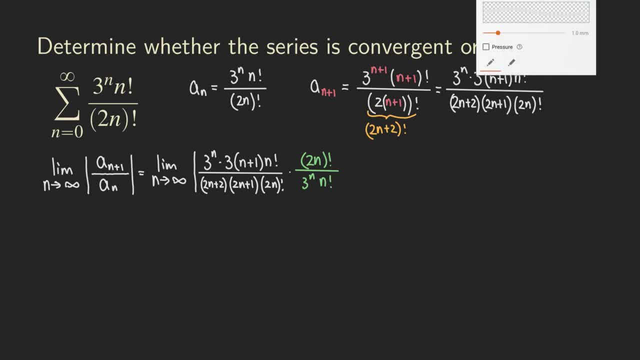 then in factorial, so that now we have the absolute value, i think all those absolute value symbols. if i use a line two to draw them, it looks a lot better. yeah, so that will be good. now that looks good, okay, so let's do a lot of cancellings here. so first we are. 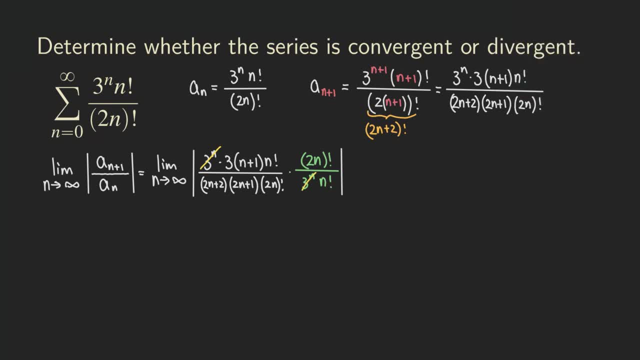 going to cancel the read to the n, and then we can cancel out in factorial, and then we can also cancel out in factorial before. so you can see right in here: much better launch, cancel the 2n, factorial. OK, I think that's it. 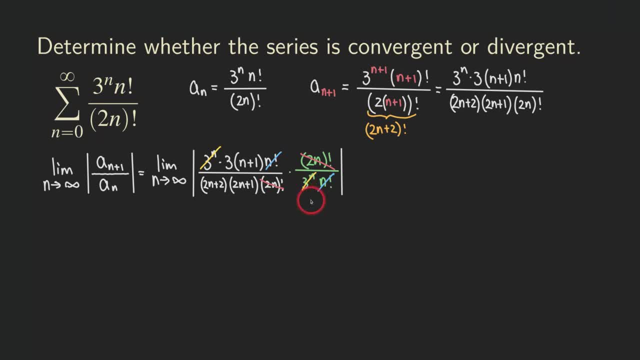 There may be more stuff that we can cancel, And I should just mention here at this point that all the factors are positive, And so we don't really need the absolute value anymore in the next step. So we are going to get n approaching infinity. 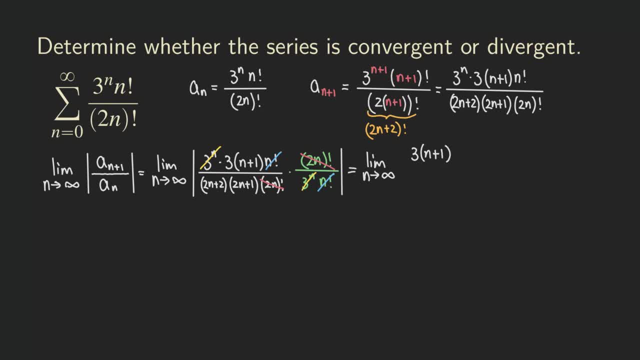 where we have the 3 times the n plus 1 in the numerator. I think that's it right. So that's it for the numerator. That's all that, And then we have what we have. Now we see that there was a 2 for the first turn. 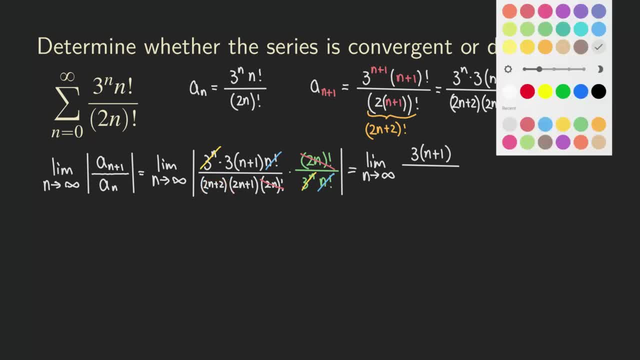 and the second turn, so we can factor the 2.. And in fact, if we factor the 2 here, we are going to get what We are going to get 2 times n plus 1.. So that means we are going to get 2 times n plus 1, right here. 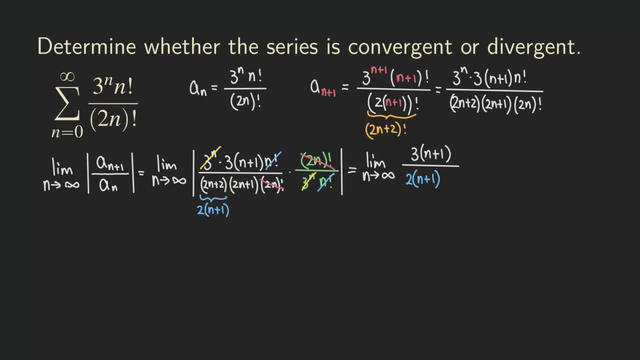 And then times what is the other, The other factor, The other factor will be 2n plus 1, right, So 2n plus 1.. OK, so that's good. We can actually just cancel one more thing right here. 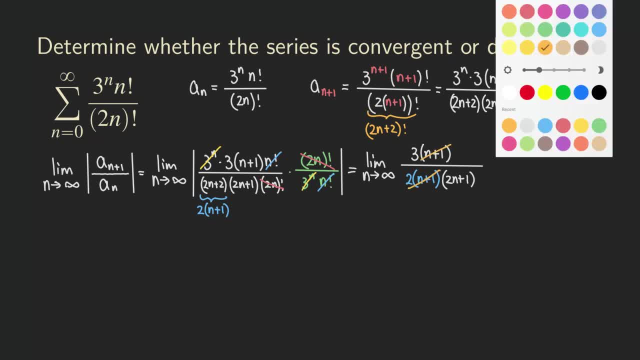 The n plus 1, we're going to cancel. OK, so now our limit actually got simplified to a really simple problem now, which is, let me see, So we are having just a 3. In the numerator, and then we have. 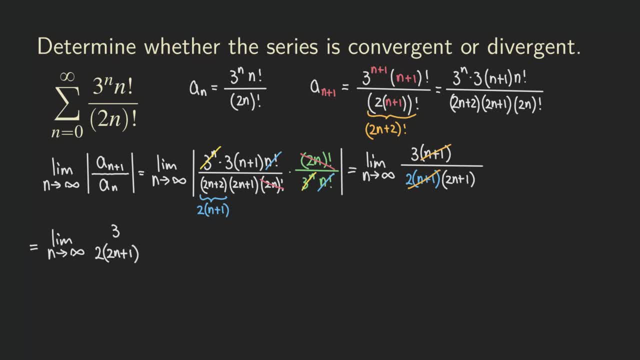 a 2 times the 2n plus 1 in the denominator. OK, so now what happens? As n goes to infinity, we have the denominator approaching infinity, but the top is just a 3. So our answer will just be 0 for this limit. 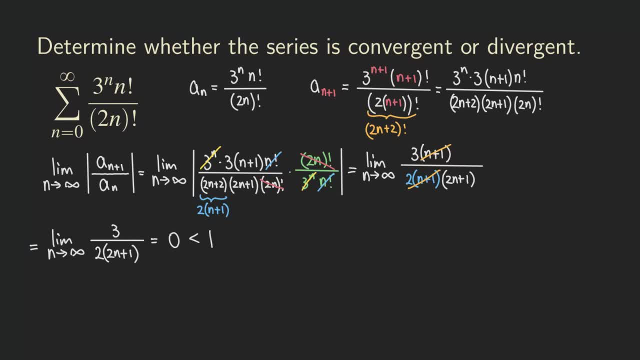 So now, since the limit of this ratio is less than 1, OK, Then we say that the series is absolutely convergent, and so it's convergent. So by the ratio, test the series 3 to the n? n factorial over. what is that? 2n factorial converges.